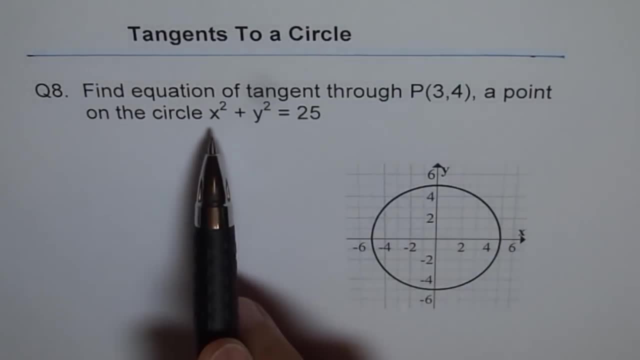 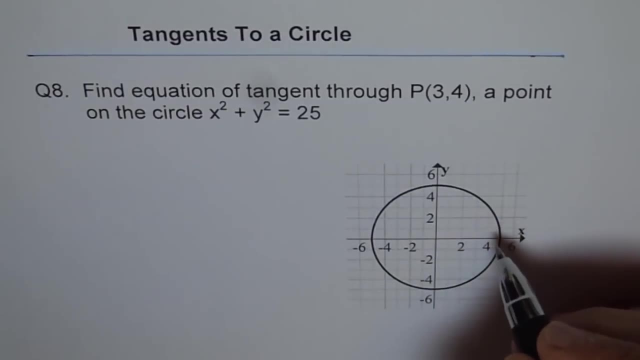 origin at 0 and radius of 5,, represented by x square plus y square, equals to 25.. The point P given to us is 3, 4, so we can plot that point on the circle. so it is 3 and 4,. 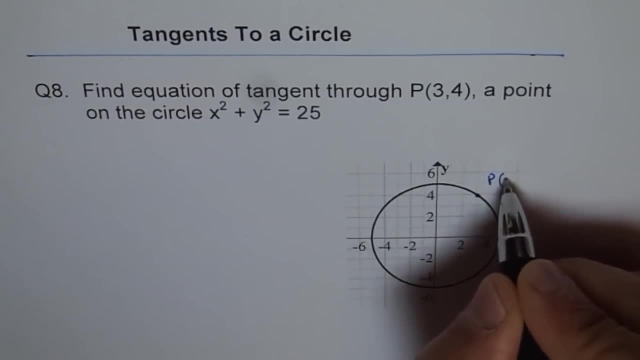 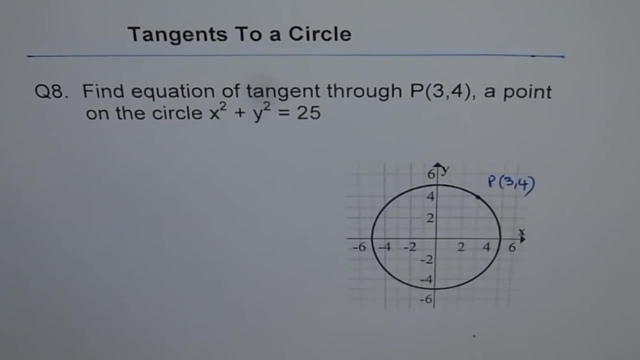 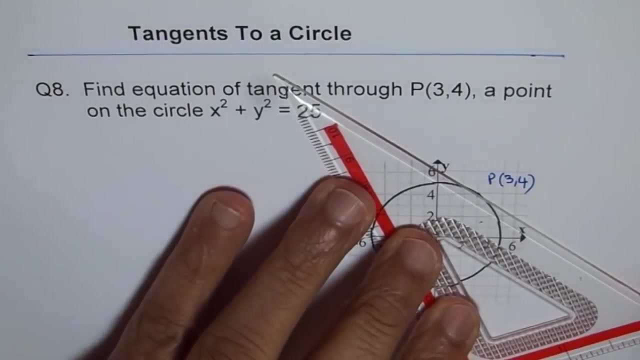 so that's the point given to us. let's say this point is 3,, 4, right, And we have to find equation of tangent through this point. So let's draw a tangent line to this point. So approximately we can draw a tangent like this: right, So that becomes the tangent. 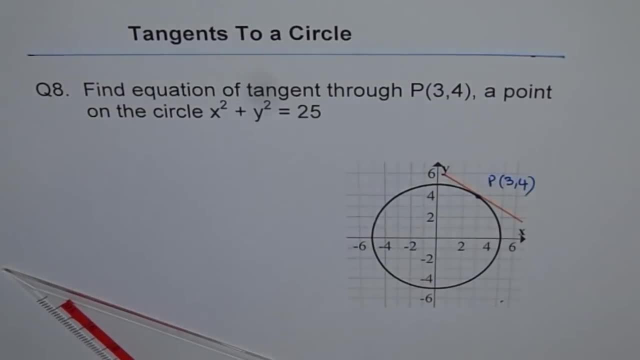 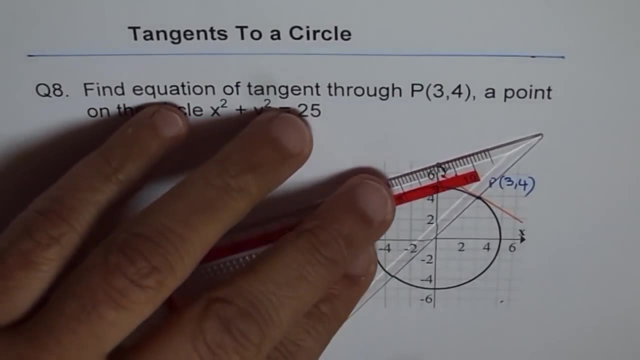 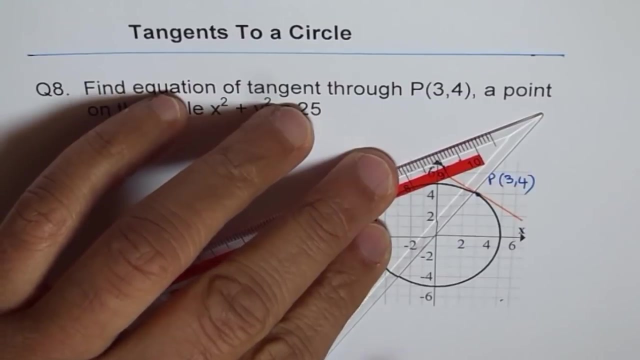 Now we'll use the properties of tangent- Tangent to a circle- and the property is that if you draw a radius at this point, then radius and the tangent, these two are perpendicular. so tangent line is always perpendicular to the radius right at this point. So if I draw this radius from here to here, then we 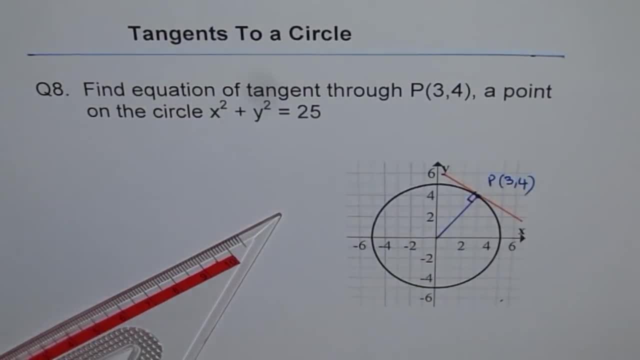 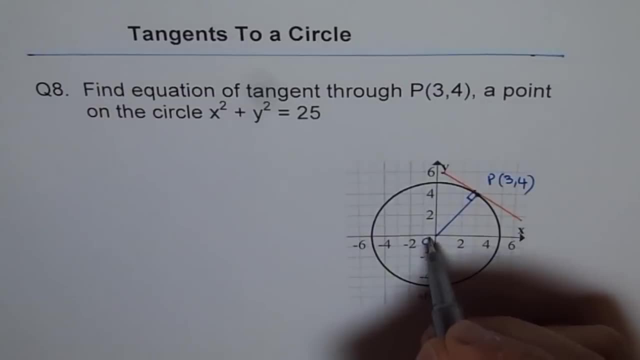 know that this will be perpendicular correct. That means I've joined this point 3, 4 with the center. So I've joined this point 3, 4 with the center. origin, which is 0, 0, right And slope of. 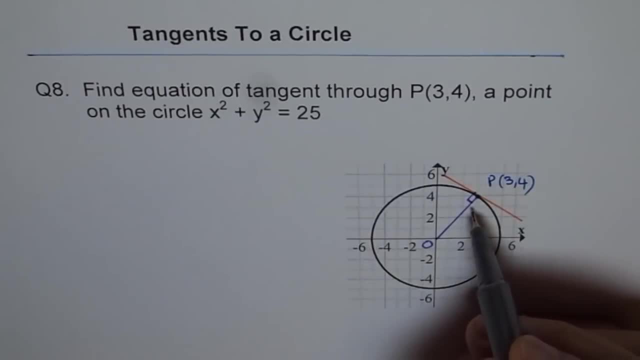 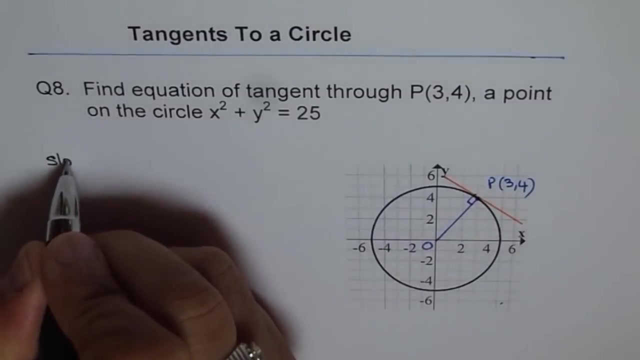 my tangent is actually negative, reciprocal of that of point O, P, correct? So that is the property of, or the relation between tangent and the radius which we are going to use to find equation of tangent line through point 3, 4.. Find slope of radius first, right. So 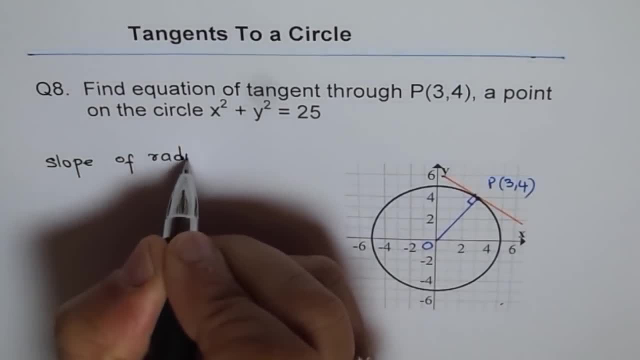 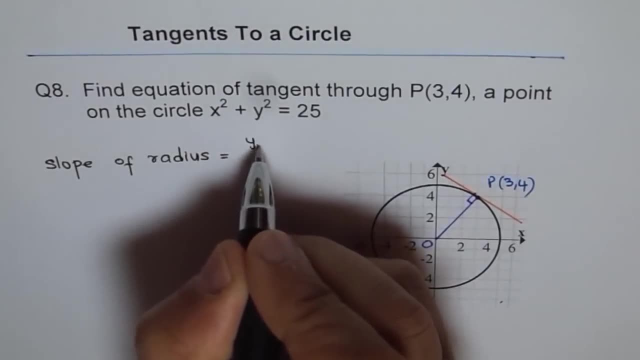 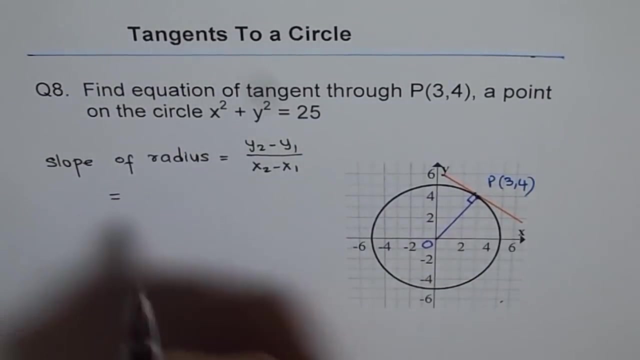 slope of radius is equals to origin, is 0, 0, and this point is 3, 4, right, So we'll use y2 minus y1 over x2 minus x1 as the slope right, So slope of the radius can be written as: y2 is 4, 4. 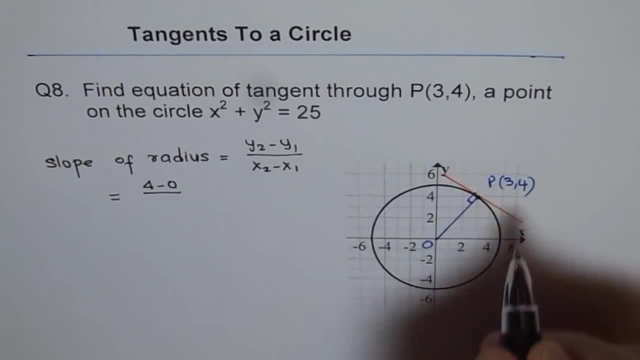 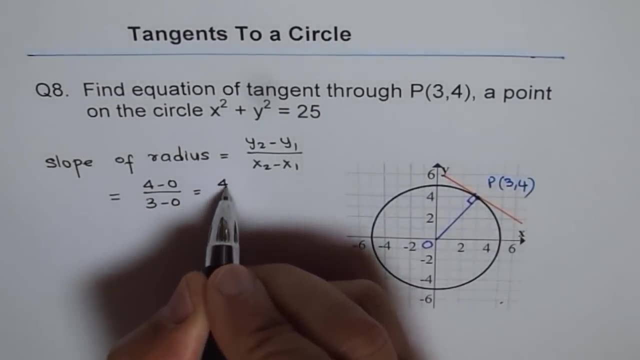 minus 0, over x2 is 3, and x1 is 0, right 3 minus 0. So we get slope of 4 over 3.. So slope of tangent has to be perpendicular, right, Negative, reciprocal. So we can write: 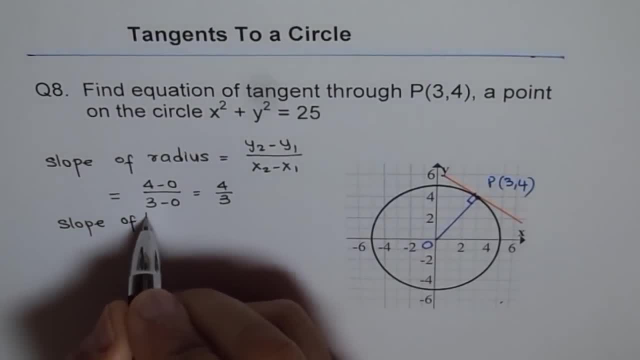 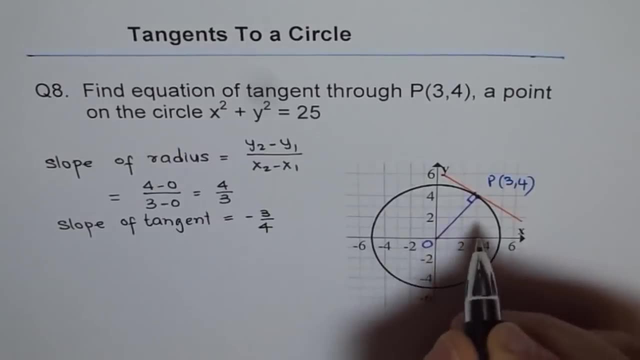 slope of tangent has to be minus 3 over 4, right Since it is perpendicular. since the tangent is perpendicular, that is the property. Every tangent to a circle will be perpendicular to the radius right, So that property we have used here. So now we know the slope of 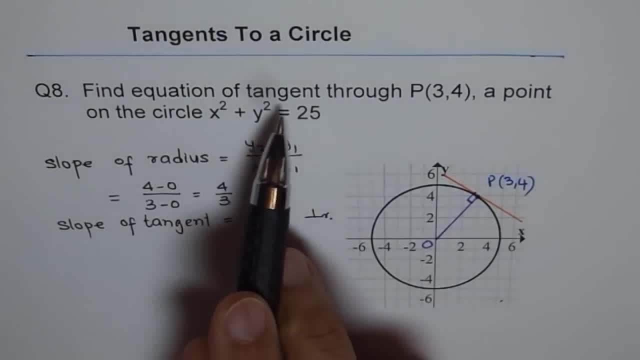 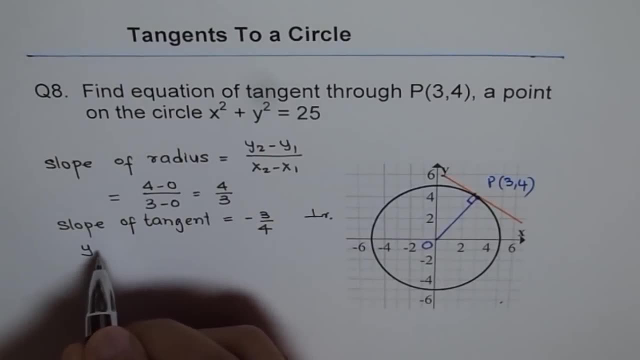 the tangent. we know the point and therefore we can find equation of the tangent right. so equation of the tangent is y equals to. so we can use either slope, intercept form or the. so we'll use slope and intercept form to find the equation of the line that is y equals to m, x plus b, right since 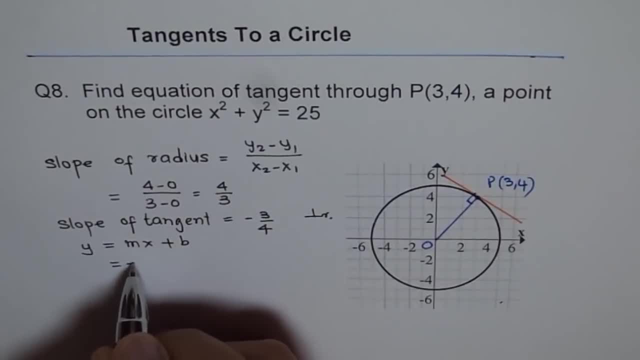 we know the slope which is minus 3 over 4. we can write m as minus 3 over 4. our point is 3: 4, where x value is 3, y value is 4, so write 4 times 3 plus b. right now that gives us. 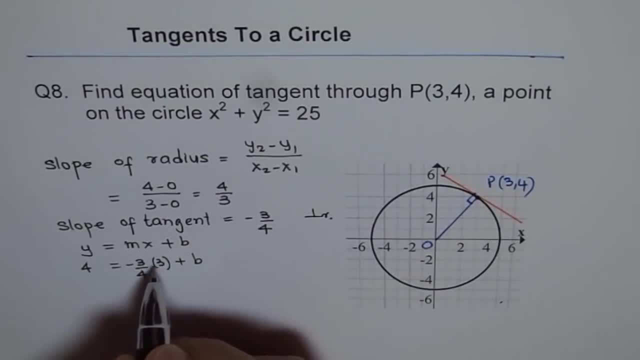 so we can bring this. this is negative 9 over 4. we can bring it on the left side and find b, so we get 4 plus 9 over 4 equals to b right and solving this we get 4 times 4 is 16, 16 plus 9. 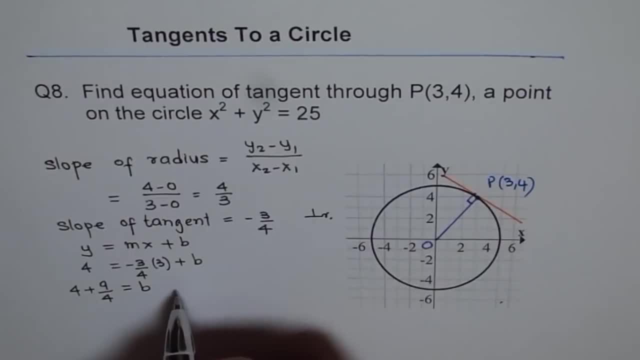 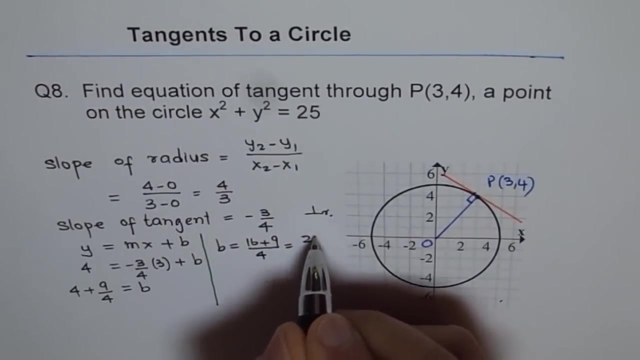 is 25, right, so we get b equals to 25. so we can write here. so we'll solve for b here, right? say: b equals to 4 times 4, 16 plus 9 over 4, which is 25 over 4, right? and therefore the equation of the line is: y equals to. 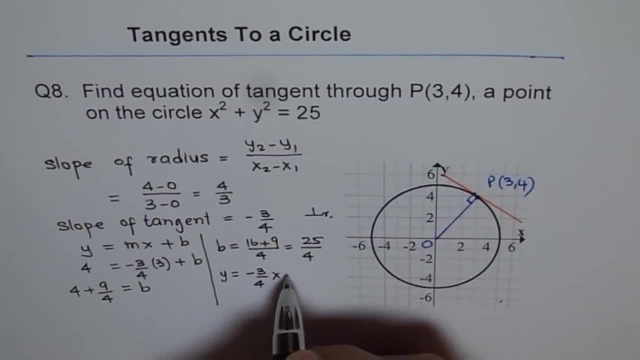 minus 3 over 4, b over 4, x plus 25 over 4, right? if you want to write this line equation in standard form, then you can multiply by 4 and then bring all the terms to one side. okay, so in that case you will get. if you multiply by 4, you get 4. y equals to minus 3 x plus 25, and bringing terms: